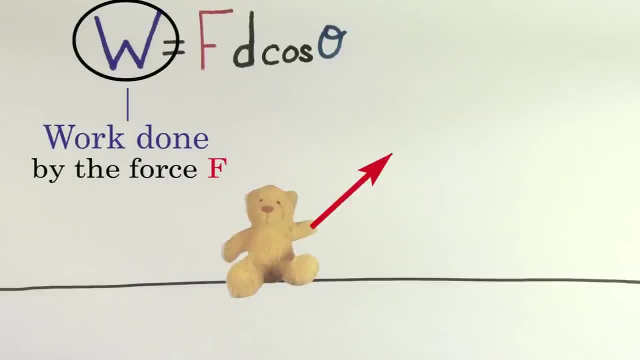 W refers to the work done by the force F. In other words, W is telling you the amount of energy that the force F is giving to the object. F refers to the size of the particular force doing the work. D is the displacement of the object, how far it moved while the force was exerted on it. 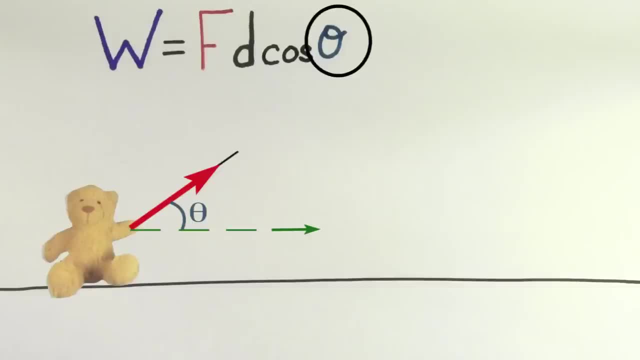 And the theta in cosine theta refers to the angle between the force doing the work and the displacement of the object. You might be wondering what this cosine theta is doing in here. This cosine theta is in this formula because the only part of the force that does work. 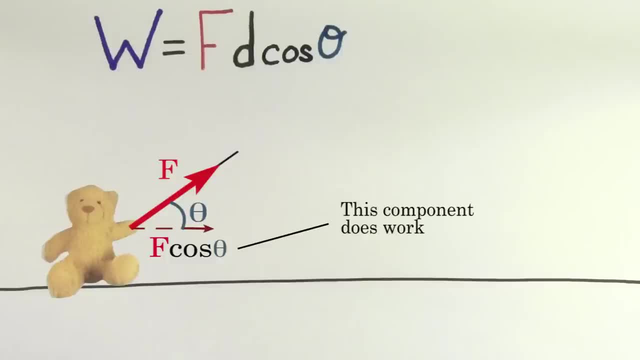 is the component that lies along the direction. The component of the force that lies perpendicular to the direction of motion doesn't actually do any work. We notice a few things about this formula. The units for work are Newtons times meters, which we call joules. 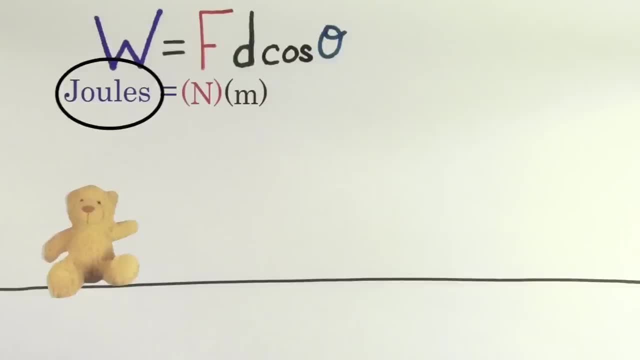 Joules are the same unit that we measure energy in which makes sense, because work is telling you the amount of joules given to or taken away from an object or a system, If the value of the work done comes out to be positive for a particular force. 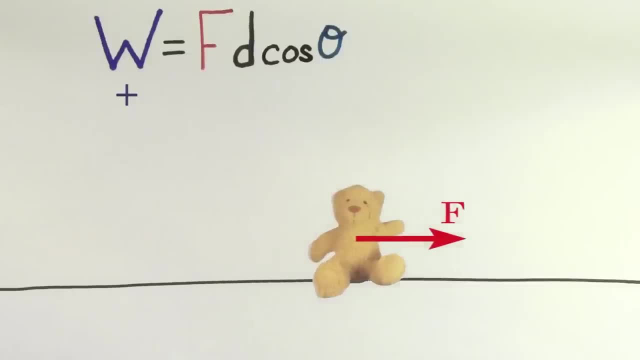 If the value of the work done comes out to be positive for a particular force, it means that that force is trying to give the object energy. The work done by a force will be positive if that force or a component of that force points in the same direction as the displacement. 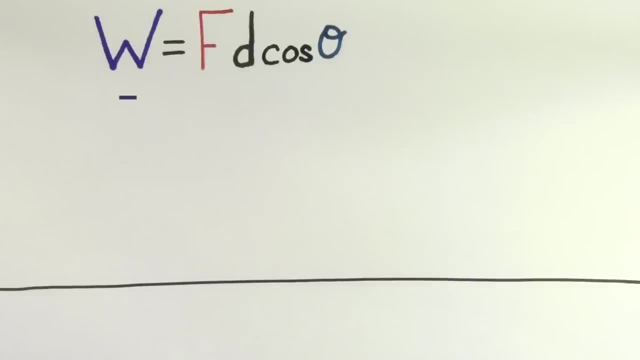